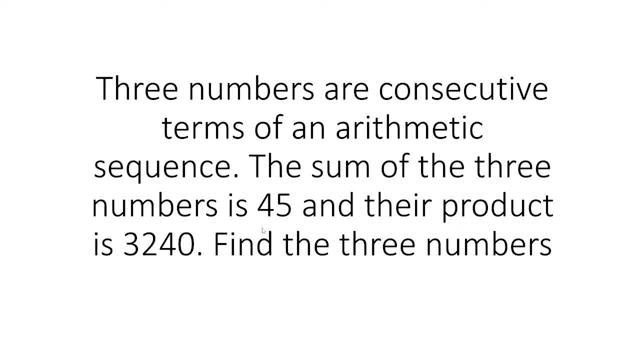 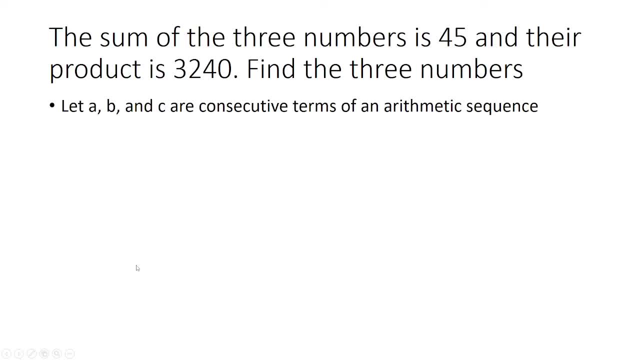 Three numbers are consecutive terms of an arithmetic sequence. The sum of the three numbers is 45 and their product is 3,240.. Find the three numbers. So we're going to say A, B and C to be three consecutive terms of an arithmetic sequence, And so when we find the sum of these, A plus B plus C, we get 45. And we multiply them we get 3,240.. So this is what is given to us. 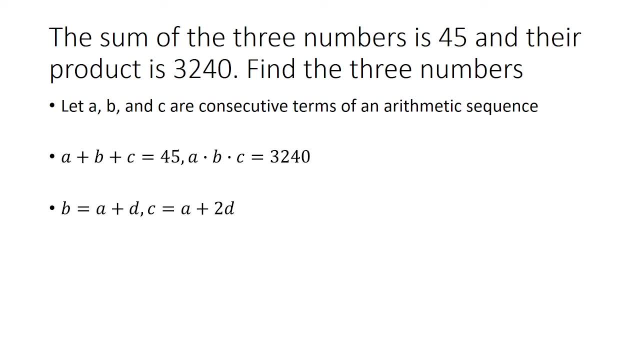 Now, because A, B and C are consecutive terms of an arithmetic sequence, we can write them in terms of the original or the first quote-unquote term with a common difference. So just for this problem, we're going to assume that A is less than B is less than C. So in order to get B from A, you have to add a common difference, So B can be represented as A plus D. 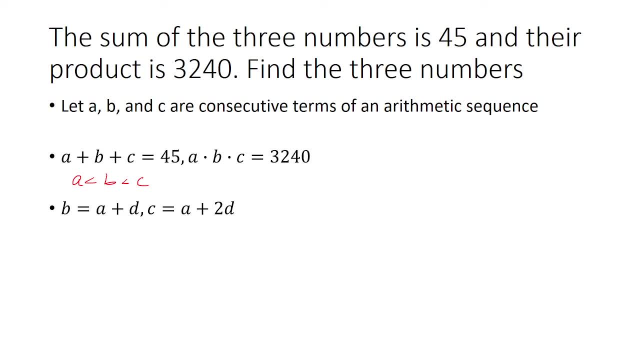 And because C is greater than A and B, C is going to be A plus 2D. So now I can replace this equation over here with these two. So we have A plus D plus A plus 2D. That's going to equal 45. So that is 3A plus 3D is 45. And if we divide both sides by 3, we get A plus D is 15.. 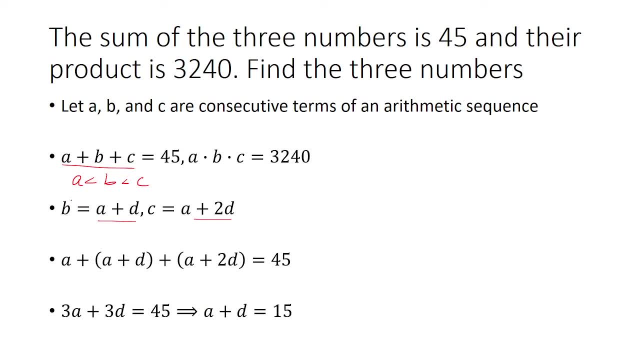 And A plus D turns out to be B. So that's this over here. So this guy is going to be B. So really, what it comes down to is finding. if we can find the common difference, we're good to go. Okay, so we just said that A plus D is 15.. So now we're going to plug that into the product. So remember, the product is 3,240. 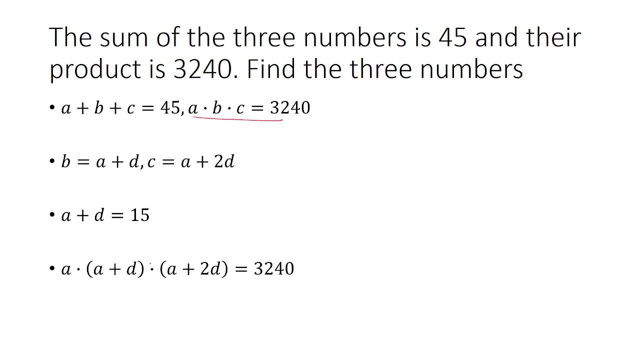 So instead of B and C, we're going to have A plus D and A plus 2D. So we're going to write A plus 2D as just A plus D and then plus D, Because I want to take advantage of A plus D being 15.. 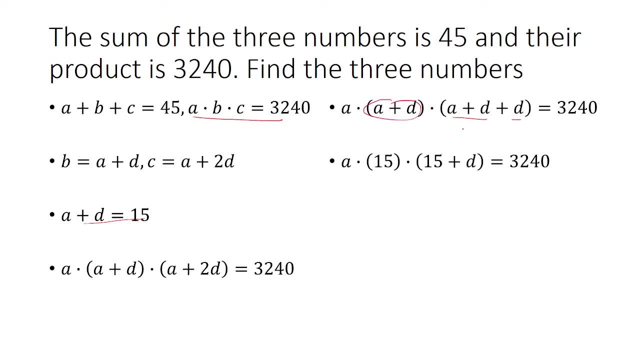 So in both of these parentheses A plus D is going to be 15.. So if A times 15 times 15 plus D, that is equal to 3,240.. We can divide both sides by 15 and then distribute the A to both the 15 and the D. 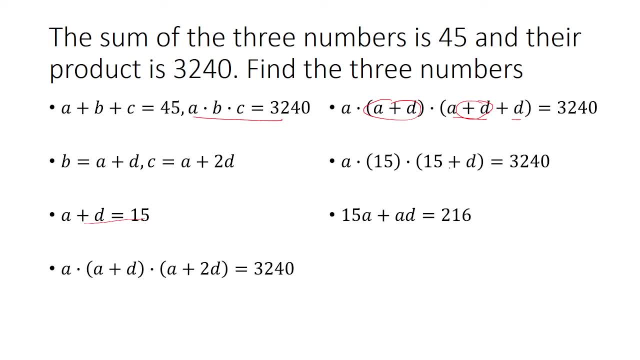 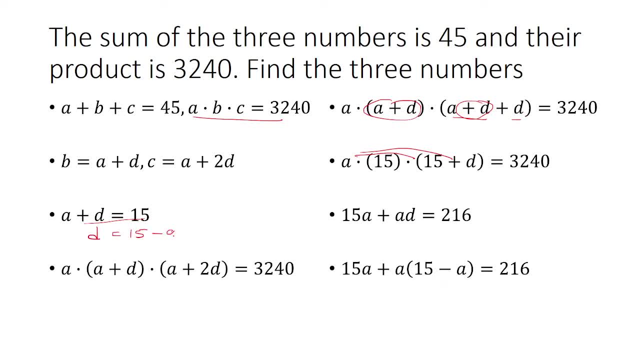 So over here we have A plus D. So over here we have A plus D is 15.. So D is 15 minus A And that goes in over here for D. So this is what we found so far And this is where we left off. 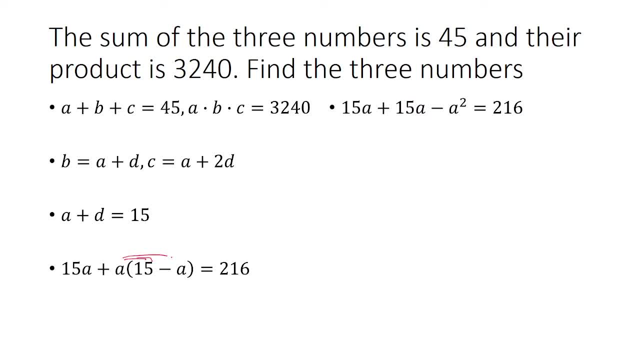 So what I did here is distributed the A to both the 15 and the negative A to get 15A plus 15A minus A squared equals 216.. Bringing everything into the left, Combine like terms, We end up with negative A squared plus 30A minus 216.. 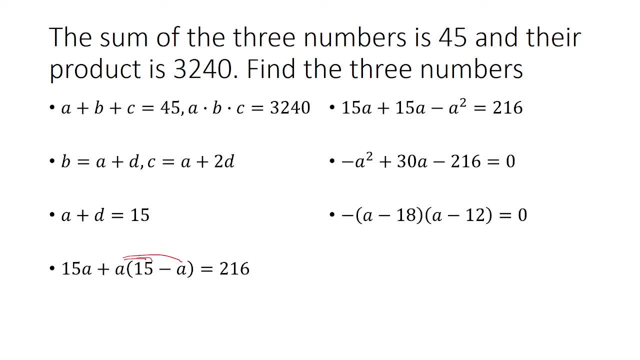 From here I can factor this out into first factor on negative 1.. And then we have quantity A minus 18 times quantity A minus 12. Set both factors equal to 0 and get A is equal to 18 and 12.. So now we get two answers. 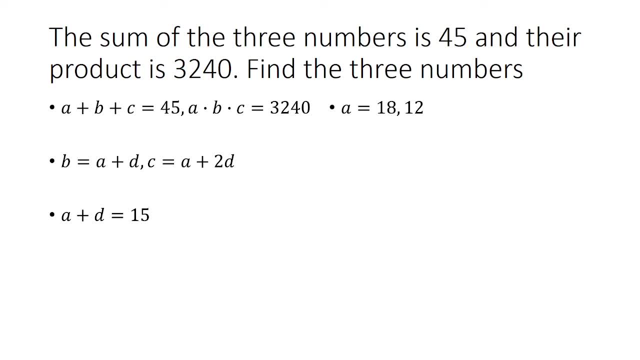 So which one is it? Well, let's go back over here. Remember this was B. A plus D is 15.. That's B. If we plug in, A is 18. Then you have A being greater than B, Which we assumed that was not the case. 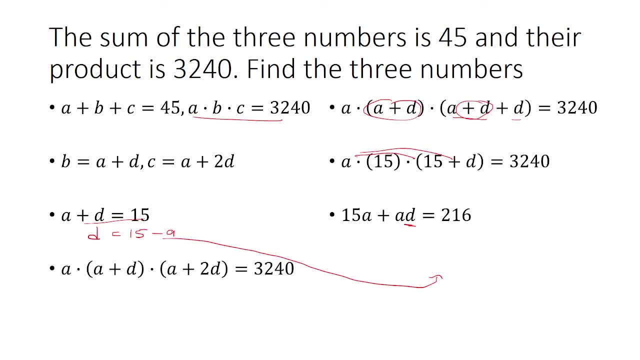 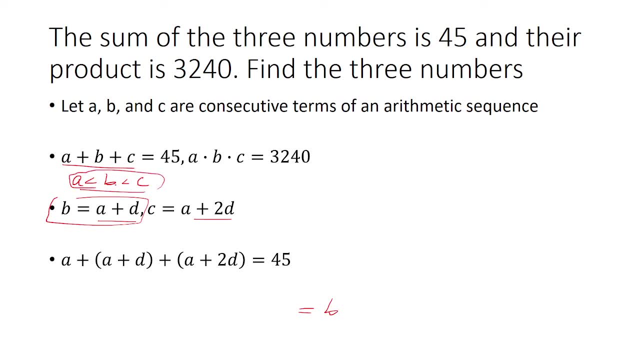 So if we go back here, We assumed that A was less than B, So that would not work. So therefore we'll say that A has to be 12.. Now, if A is 12. D has to be 3. So then we go over here.